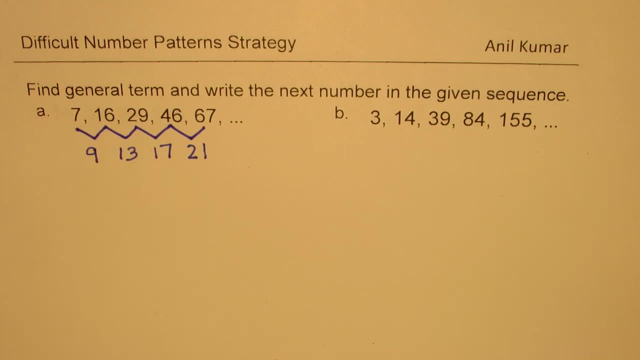 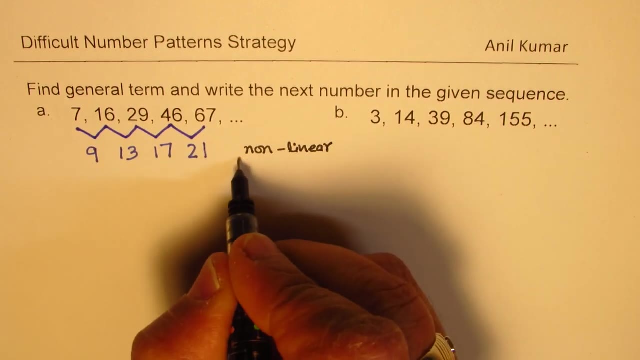 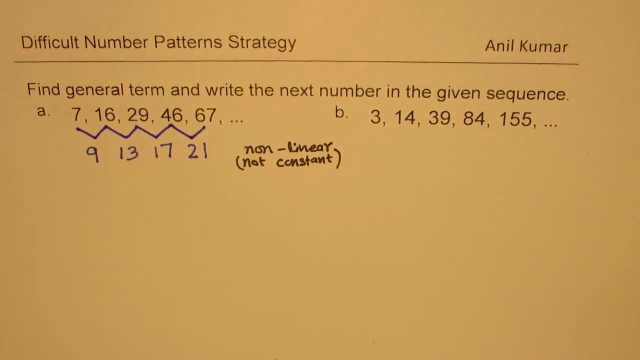 So let me write down here. So here the difference: it not constant, So that means nonlinear Since it is not constant, Correct. Now if I continue this pattern and find the second difference, then what do I get? Well, second difference in this particular case is is 4.. 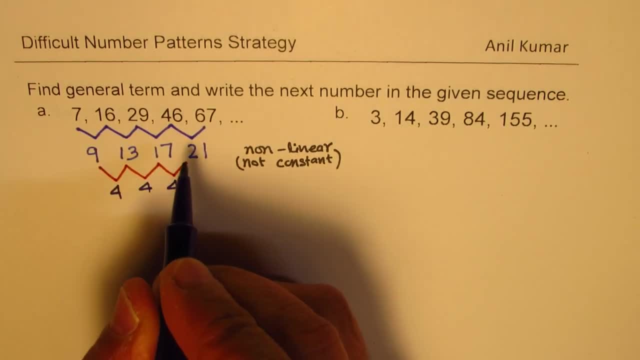 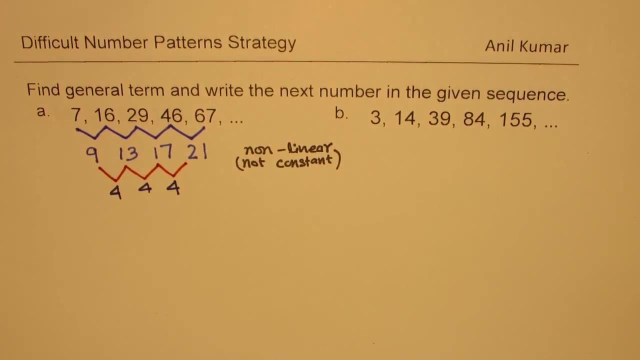 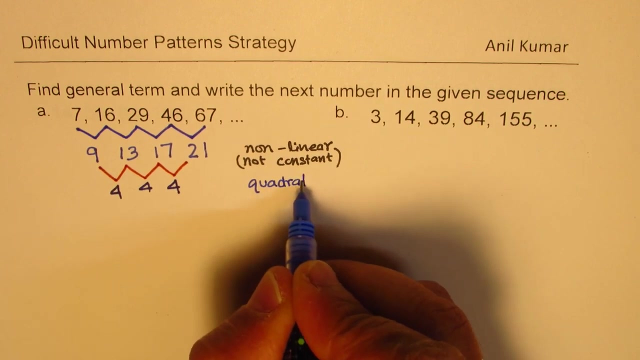 Here also, it is 4 and 4.. If I do 4, I get 8.. correct, so that means we have a second difference of 4 that means it is: this is constant. that means it is quadratic. is that clear to you? perfect now the 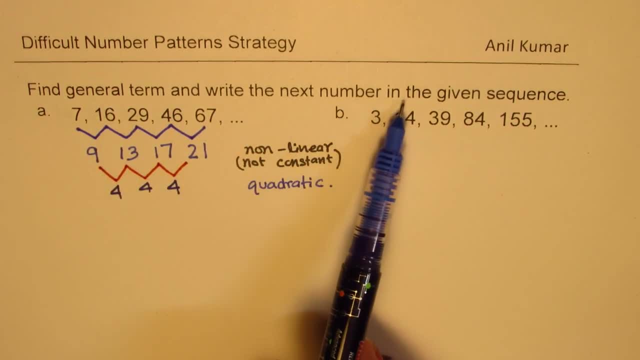 question is: find the general term and write the next number in the given sequence. now, since we have to find a general term, we will really have to explore and figure out how to get the general term. sometimes, the question is only to find the next number. that was simpler, because what we could do here is: 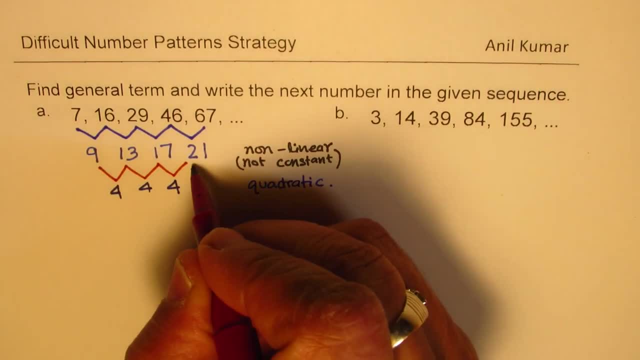 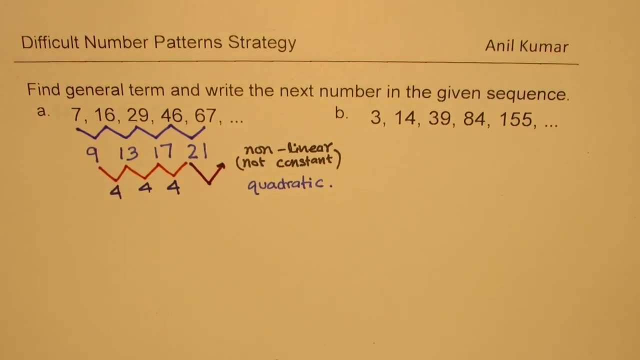 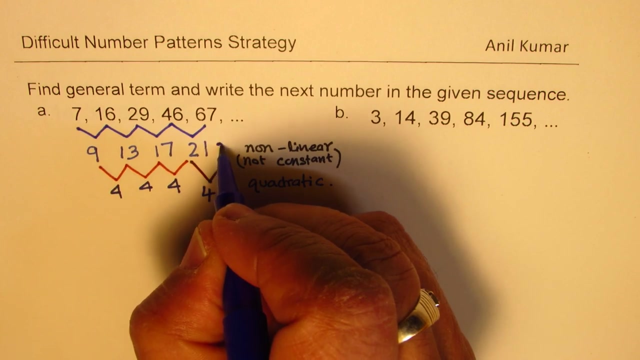 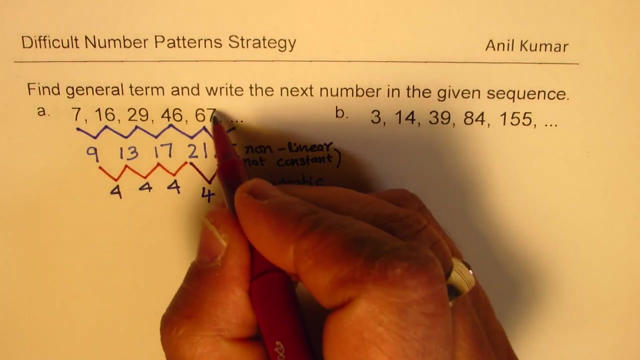 that we could just continue with this, and we know the next number here you can get by adding 4, correct, so. so if you add 4 to this, right so, and then 21 plus 4 will give us 24, 5, and then you can add 25 to get the number here right. so 5 plus 7 is 12, 2, and 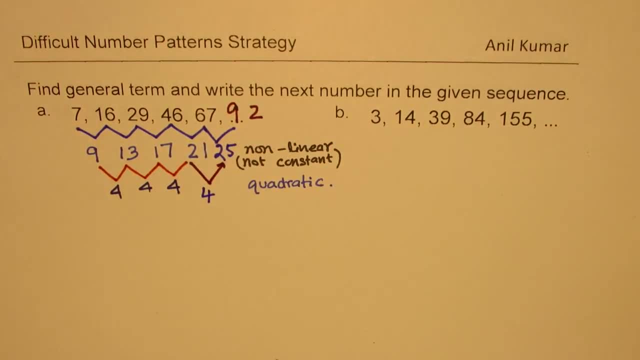 1, 92. so the next number is 92. so if the question was only to find the next number, you could have done this. however, it says find the general term. so how do we do this? so one thing is clear: it is quadratic. that means in our set of: 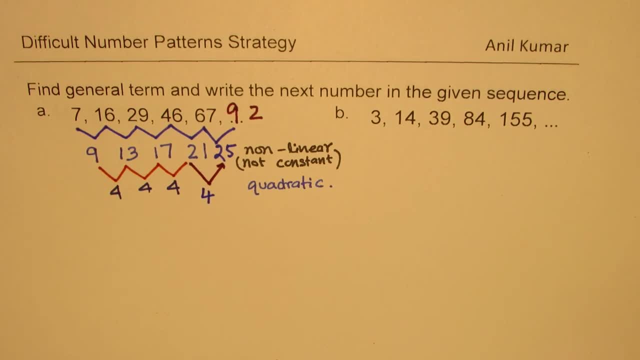 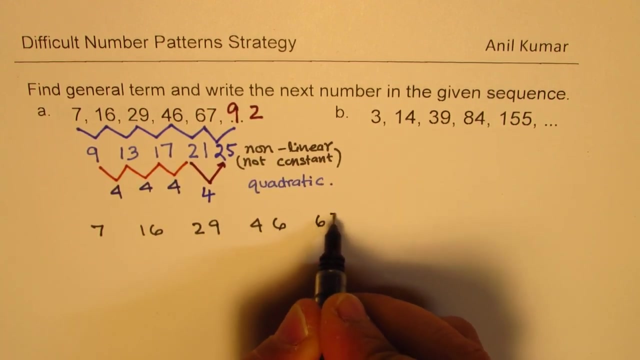 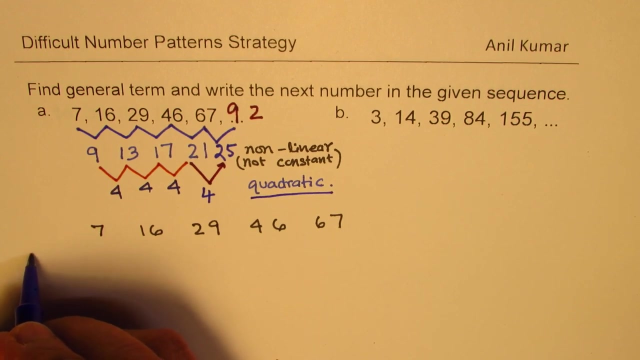 numbers. n squared is definitely related some way or the other, right so? so we could actually write this as 7. we'll again begin with exploring more about this particular sequence, which is- I'm just writing this down- 67, 3. so what we will do here is that, since it is quadratic, we'll write down the powers of numbers. 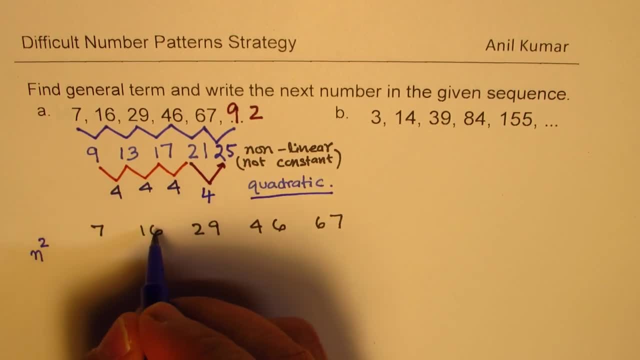 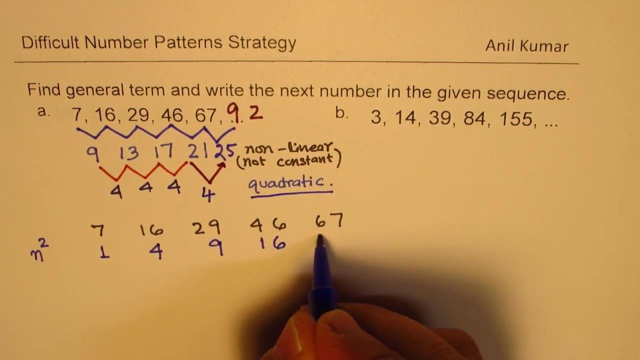 right n squared. so this is my first term, this is my second term, so I write here 1 square, which is 1, and there I am writing 2 square, which is 4, and 3 square, which is 9. 4 square is 16, 5 square is 25, so when I have written, 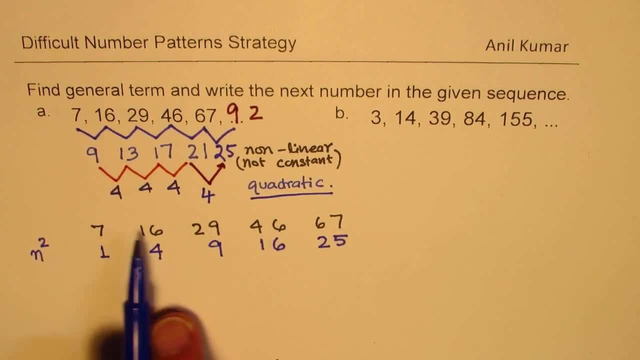 these powers. I still say that to get the number 7, 16, 29, what we could do is we could actually further explore and find their differences, so we can actually do this right. so let's find their differences. how much do we add now to get our 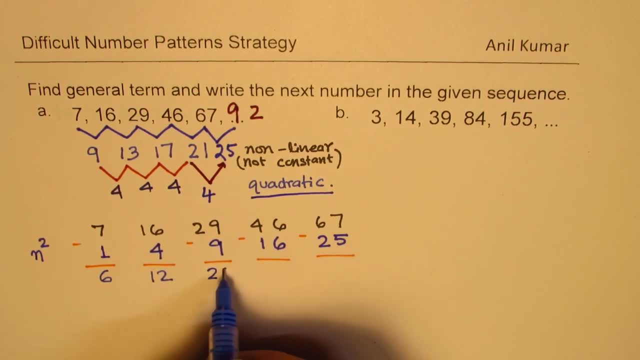 original number. that is what the strategy is. so 7 minus 1 is 6, and 16 minus 4 is 12, 29 minus 9 is 20, 46 minus 16, that is 30, and when you take away 25 from 67 we get 42. so we get the sequence of 612- 23, which is the number 3 on the 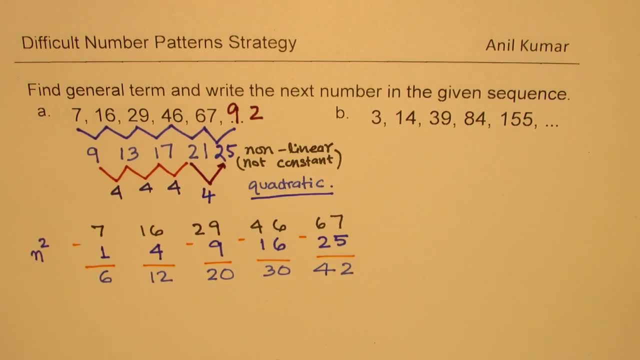 30 and 42.. Now this is kind of very important and familiar sequence for many who are exploring this series of, you know, patterns, number patterns, correct. So what you notice here is that you could write 3 as this number, 6 as 2 times 3. you can write this as 3 times 4, right? So this is 2. 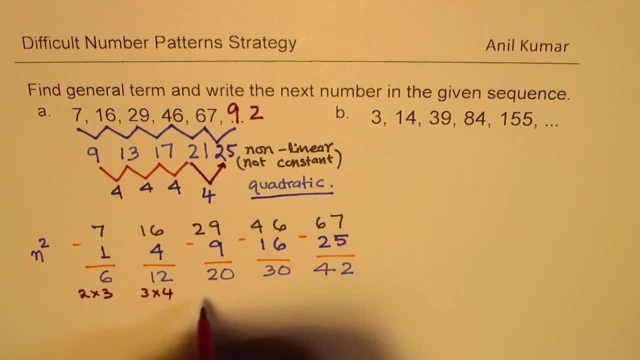 times 3, and this is 3 times 4, and this is 4 times 5, and that is 5 times 6. this is 6 times 7.. So you do see a pattern. do you see that correct? Now, if you look into the term numbers, right, let's. 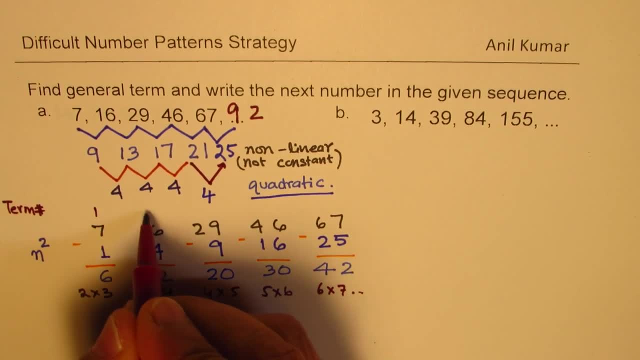 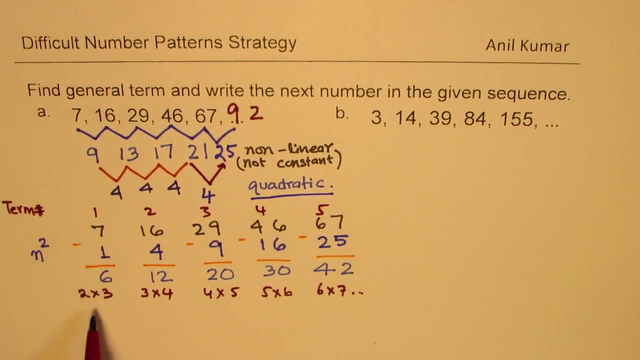 write the term numbers. So this is term number 1, 2, 3, 4, 5 and so on. So, looking into this, you can now find a general term, right, So we can write the general term tn as equal to. first we need this 1 and then we need this 6 to get 7.. 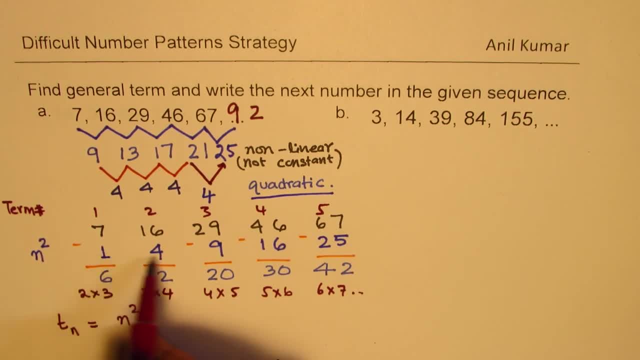 So it is n squared right. So that is gives you 1, 4, 9 and all plus this sequence right 2 times 3.. Now 2 is 1 more than 1.. So we'll write this as n plus 1 times n plus 2.. Does it make sense to you? 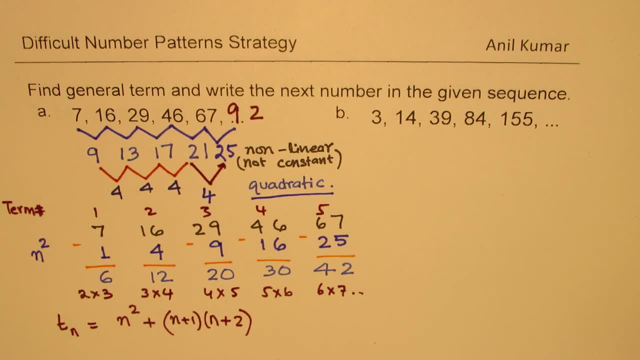 Correct. So that is how you can write the general term tn as equal to 1, and then we need this 6 to get 7.. Now you could get your general rule very easily, without really getting into polynomials and their equations. Now some of you who are familiar with polynomials- let me write down: Well, actually have 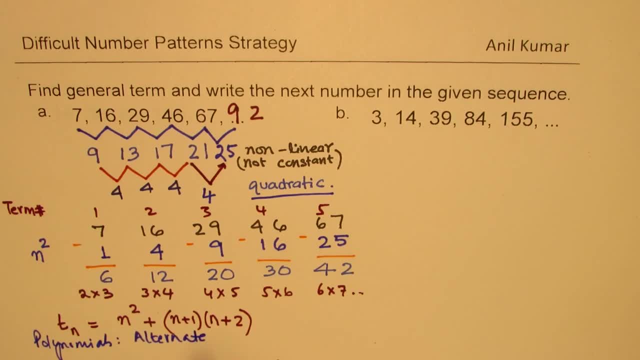 an alternate method. right, and since we know that the second difference is 4, we could write: a is 4 divided by 2.. So we can write: a is 4 divided by 2.. So we can write: a is 4 divided by 2.. So we can. 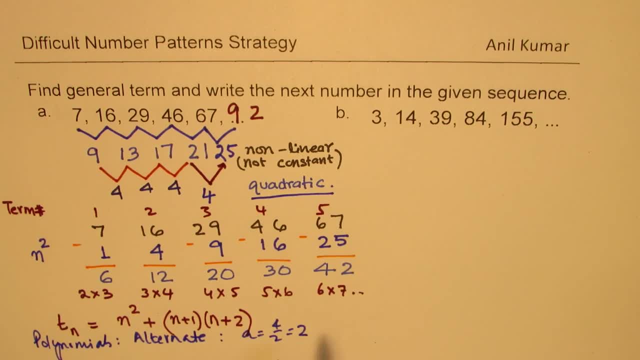 write a is 4 divided by 2, which is 2. right and though, so we could actually get alternately using a as 2, our answer, but I'm not getting there correctly, So I hope this helps you to understand how we could actually get a pattern using this. 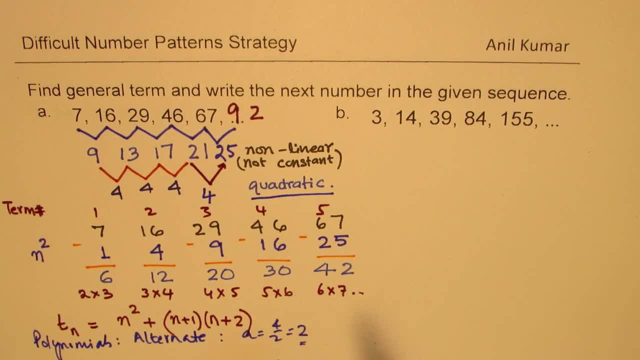 method correct. So I like you to know, explode the second series, which is 3, 14, 39, 84, 155, and get your pattern, which is very similar to this one, right. so once you explore, I'll share with you the solution for the second series also. so let's move. 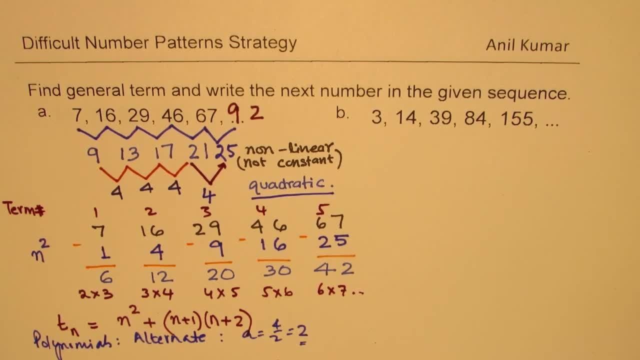 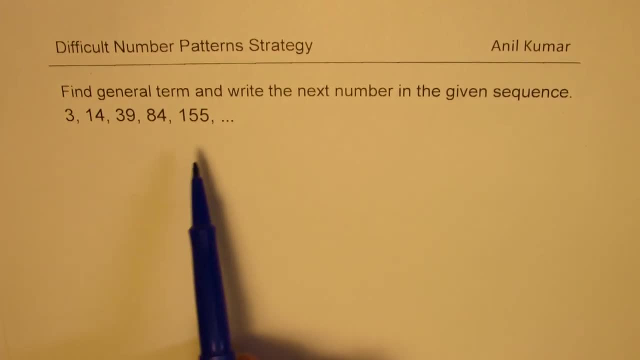 forward and see how we can solve the second related series. now let's take up the next example. we need to find a general term and write the next number in the given sequence: 3, 14, 39, 84, 155 and so on. so the numbers are really going up. 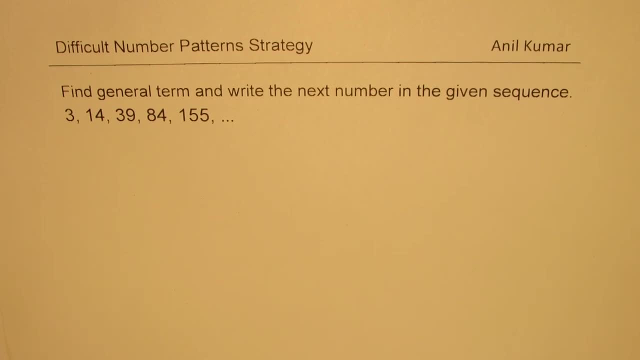 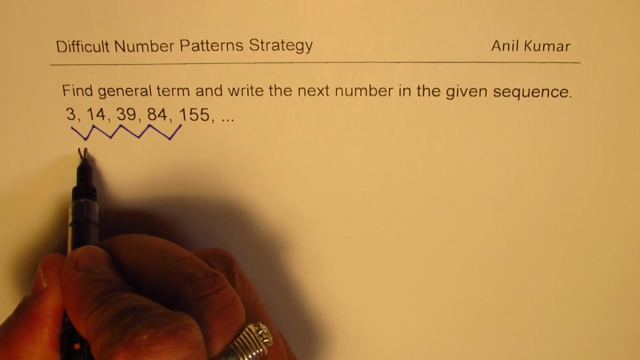 very high, so it has to be n to the power of something, right? let's find the difference. so let's start with finite difference, which is a very standard way of solving such questions. so we need to 14. take away 3, what you get is 11 and 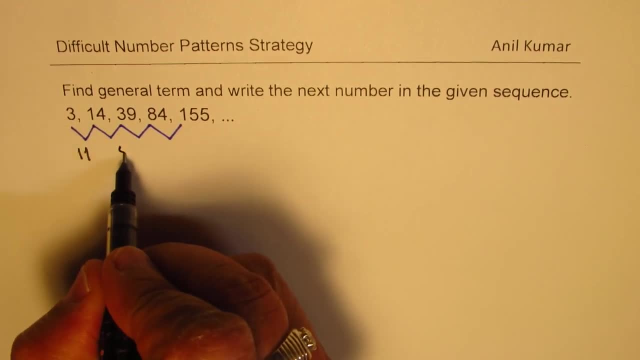 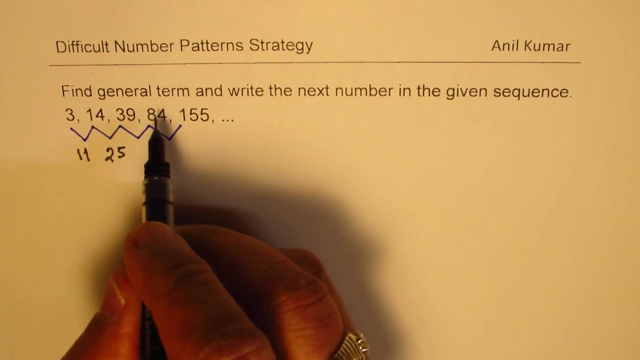 here: 39. take away 14, we get 5, and 9. take away 1,. 3. take away 1 is 2,, 25.. 84, when you take away from 14, you get this number as 5, and 7. take away 3 is 4.. 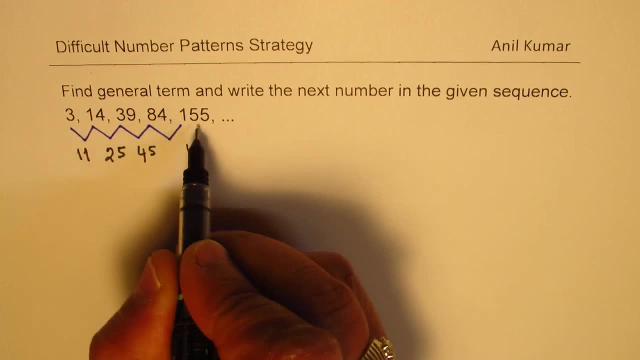 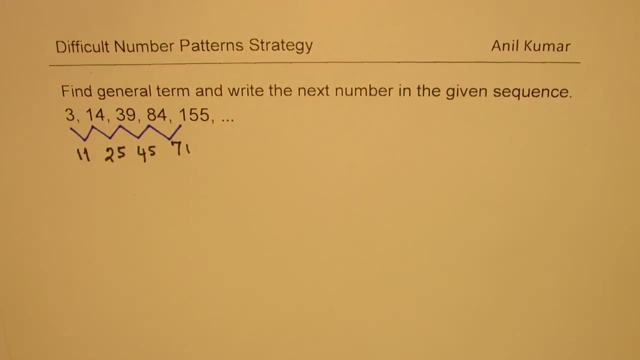 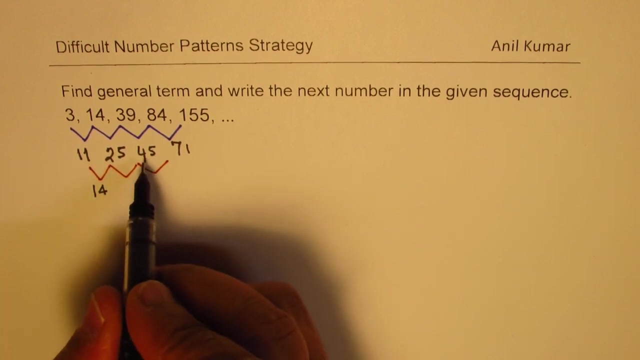 155,. when you take away 84, you get 1, and 15 gives you 7 here, right, So you get 71.. Definitely it is non-linear, so we'll go for the second set of difference: 25 take away 11 will give us 14, and now this gives you 0,, 20, and here we get 11. take away 5 is 6,, 26,, correct. 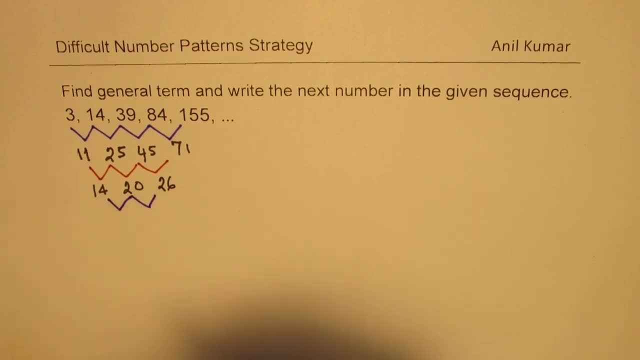 Now another level gives us 11. A difference which is constant and which is 6, correct? So that means we are looking into a cubic relation. Do you see that? So we are looking into a cubic relation, Since third finite difference is constant. 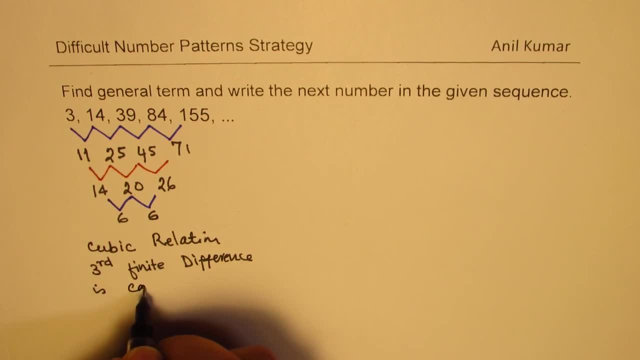 is that clear, Right? So that is what we are looking into Now. some of you will know that this relation, a, the leading coefficient, will be 6 over 3, factorial, which is 1,. right? So you know that the relation will be: y equals to a is 1, so it will be. you can write in terms of n, the term numbers, n, cube plus, so on. 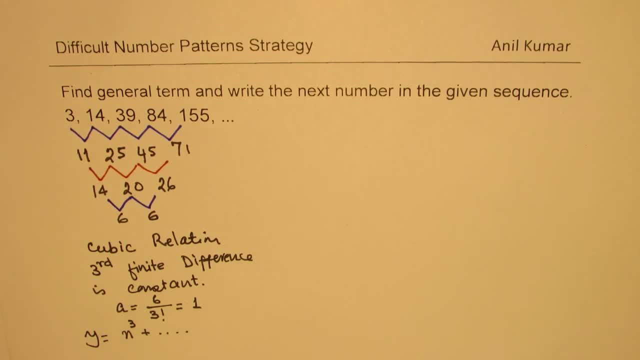 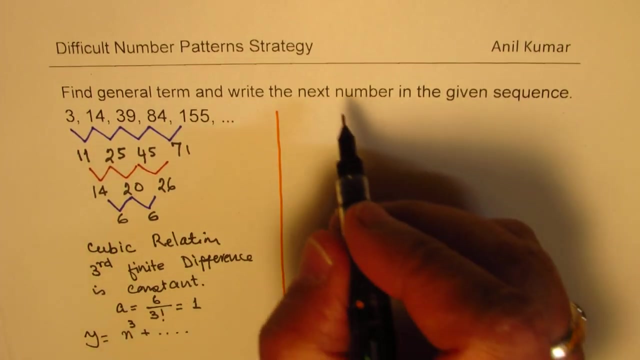 Right? So here is a shortcut method to find how we can. We could get the other terms and get a general term for this particular sequence. So let's try to analyze it just as we did earlier. We know that n cube is definitely a part of this relation, right? 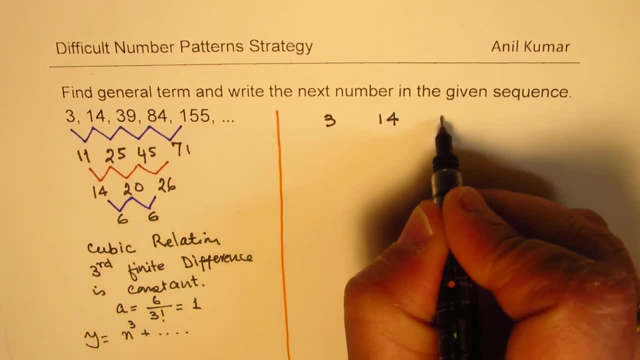 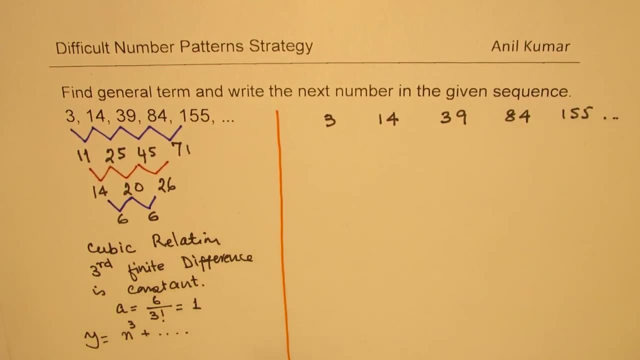 So I'm rewriting these numbers. We have 3,, 14,, 39,, 84,, 155, and so on, correct? So let's write down the cubes of numbers, correct? So let's write down the cubes of numbers, correct. 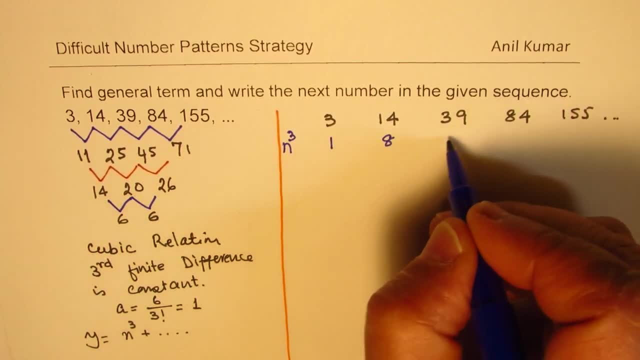 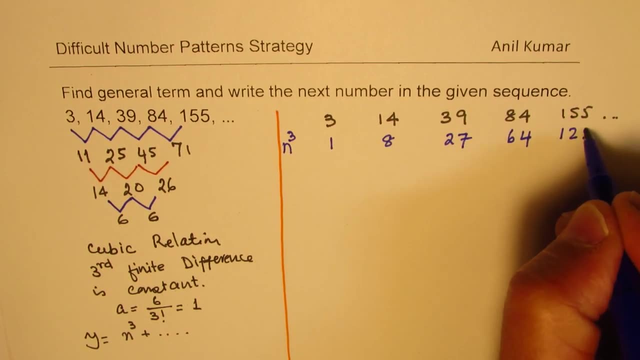 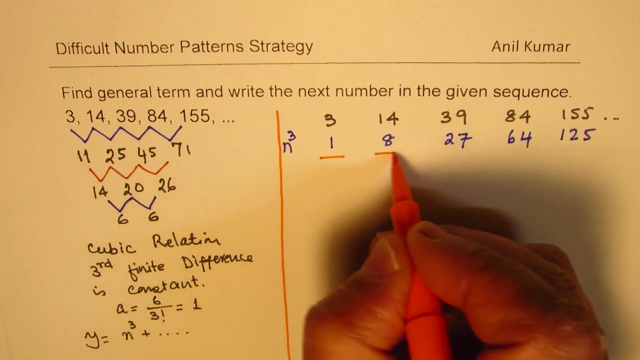 So 1 cube is 1,, 2 cube is 8,, 3 cube is 27,, 4 cube is 64, and 5 cube is 125, correct? So these are the cubes of the number. Now, if I write down the cubes, how much is still remaining? that is what we need to figure out. 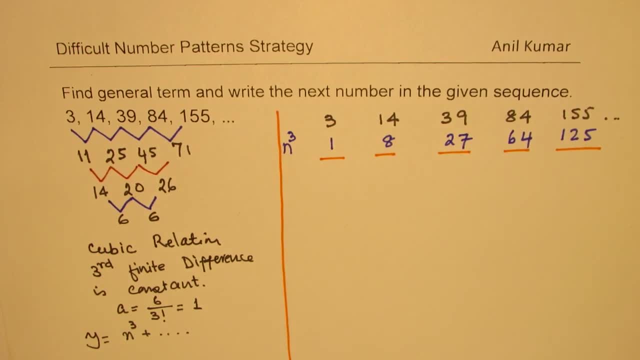 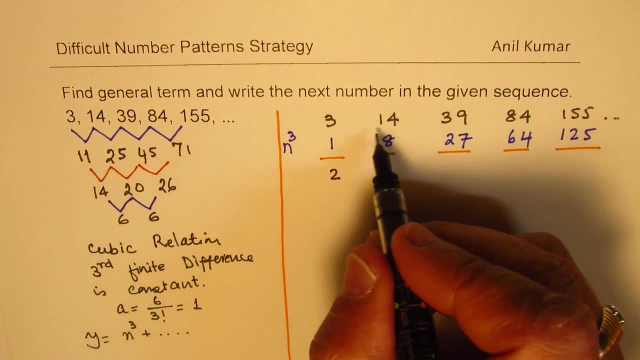 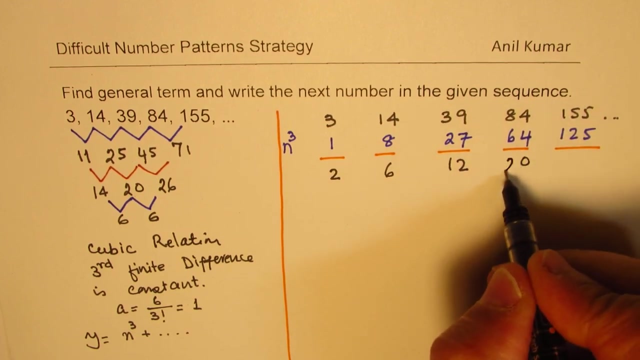 So 3 minus 1 is 2 remaining, right, So this is 3 minus 1.. So we are not taking the difference. So this one is 2 remaining, and 14 take away 8 is 6, and here we get the number 12, and 84 gives us 20, and that gives you 30,, right. 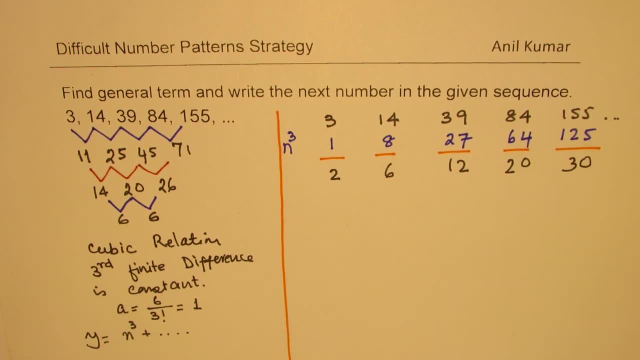 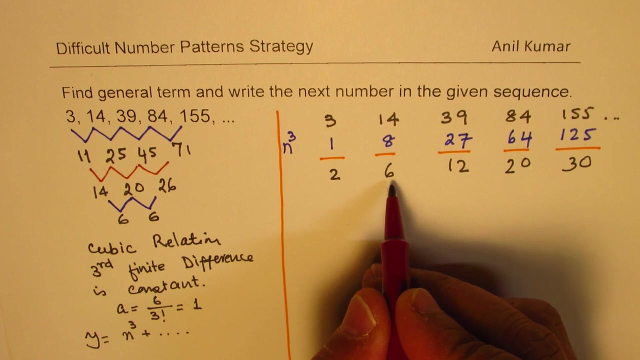 Do you see that familiar number series, right? This is a very interesting series, since that tells you that they could be written as product of consecutive numbers, right? So we can write this as 1 times 2.. This is 2 times 3.. 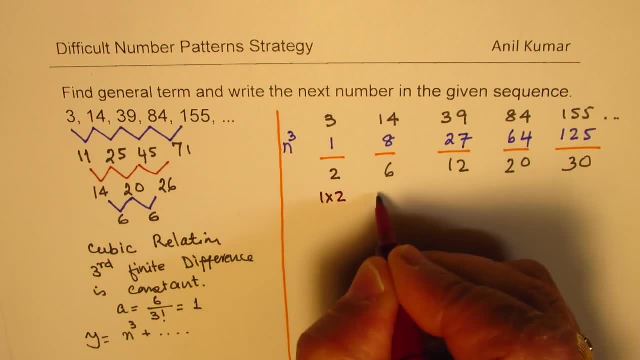 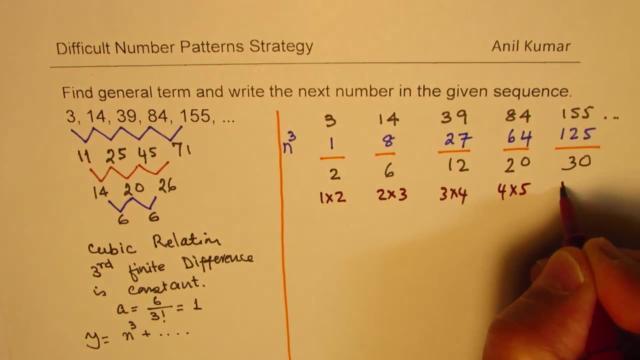 This is 3 times 4, and so on. So this is like 1 times 2.. This is 2 times 3, and that is 3 times 4.. That one is 4 times 5.. Then we have 5 times 6, and that is how the series goes correct. 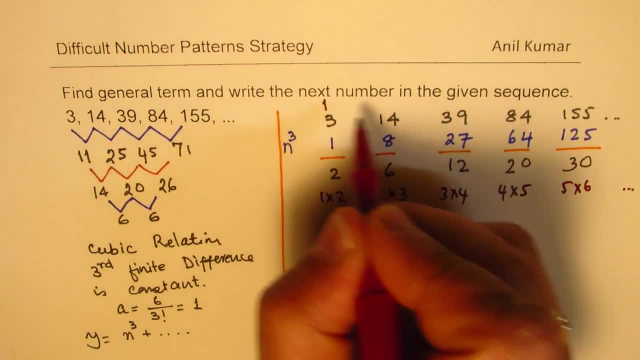 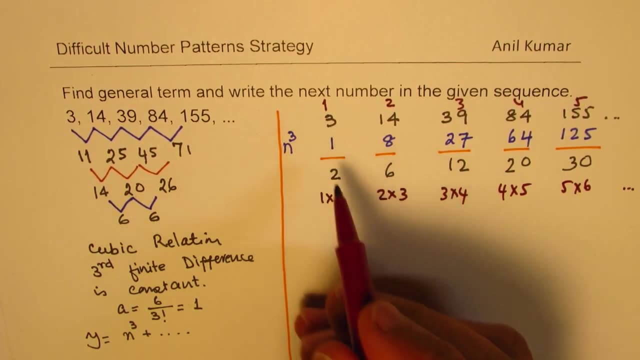 So now that gives you an idea. Your term number: this is 1,, this is 2,, this is 3,, 4, and 5, and see how they are related correct? So from here we can say that the nth term is n cubed. 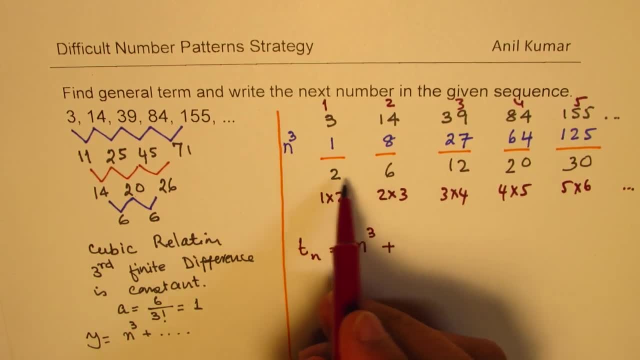 Plus, you have to add these numbers 2,, 6,, 12, which could be written as n times n plus 1.. Does it make sense to you? Correct So if you have to find the 6th term? so what you need to do here is you do 6 cubed plus 6 times 6 plus 1, and that's how you could get your answer correct. 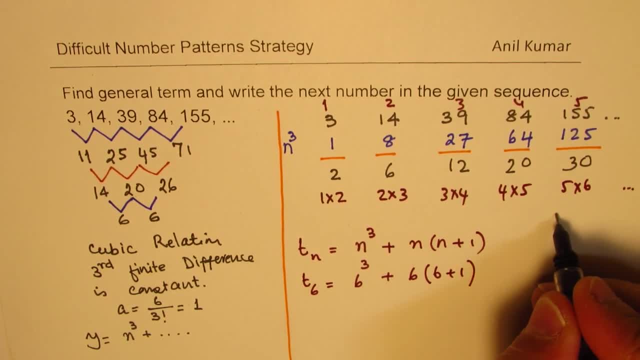 So you can do 6 cubed, which is 36 times 6.. 6 times 6 is 36,, 3.. And 6 times 3 is 18,, so it is 216.. And that is 6 times 7,, which is 42..